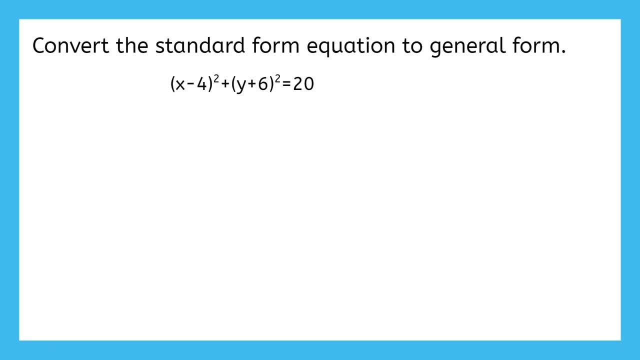 in action. In our first example problem, we need to convert the standard form equation into general form. In order to write this equation in general form, we need to expand this as much as possible. So let's start there. What is x minus four squared actually telling us to do in terms? 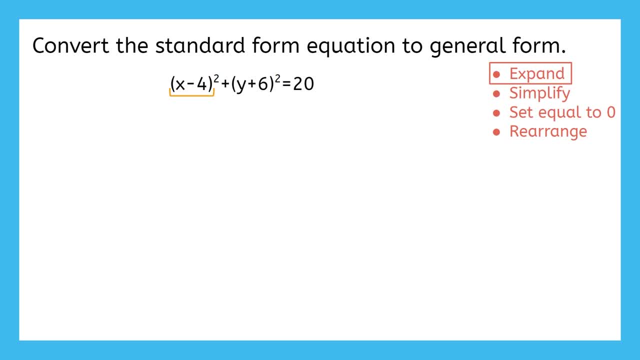 of operations. Since this binomial is being squared, it means we need to multiply x minus four times itself, which looks like x minus four times x minus four. Using this as an example, what will y plus six squared look like? Exactly, This means y plus six times y plus six. We can't expand anything else. 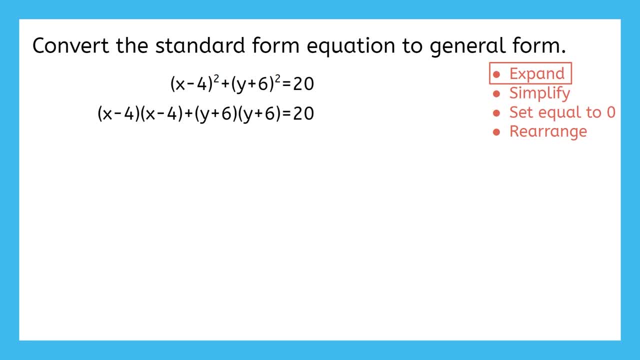 so let's just bring down the equals 20.. We can continue, Continue expanding by multiplying each pair of these binomials. Pause the video now. to multiply x minus four times x minus four and y plus six times y plus six, Your multiplication of x minus four times x minus four should look like this: I've chosen to use a. 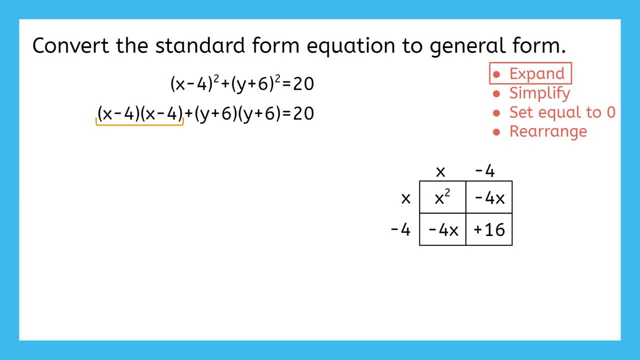 visual or area method to multiply, but if you prefer a method like FOIL, that is okay too. You should still get these same four terms. Now I'm going to substitute all four of these terms for x minus four times x minus four back into my 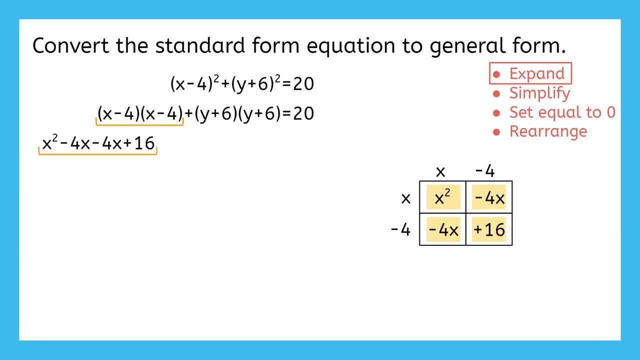 equation and worry about combining my like terms in a moment. Now we can repeat this with y plus six times y plus six. Your multiplication of y plus six times y plus six should look like this: Likewise, I will be bringing all four of these terms back into my equation. 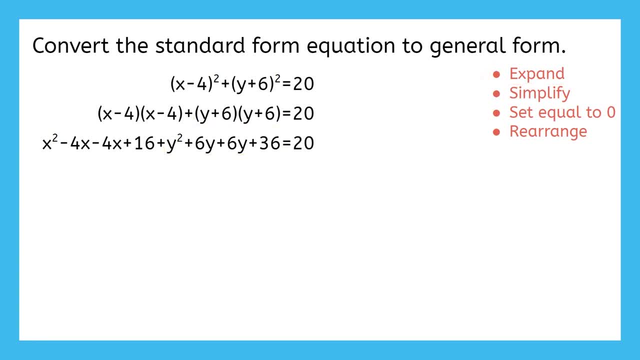 At this point, we have expanded as much as possible, but this equation is still an absolute mess. I'm gonna clear out the line that we've finished with to help make some space, and next we're going to need to work on combining the like terms. to simplify this thing, Pause the video here and combine your like terms. 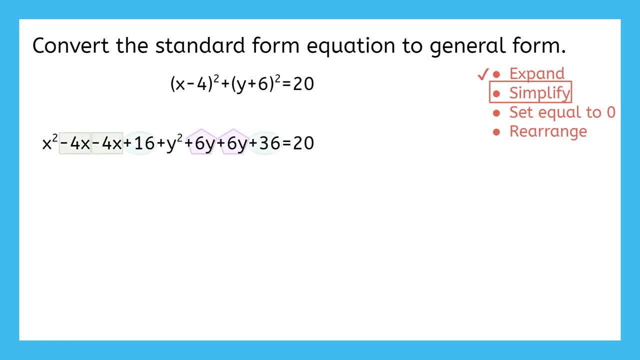 I like to color code my like terms to help me stay organized. so here are all the like terms on the left side of this equation, equation that need to be combined, And when I combine them my equation looks like this: Negative: 4x minus 4x makes minus 8x. 6y plus 6y makes 12y. And lastly, 16 plus 36 makes 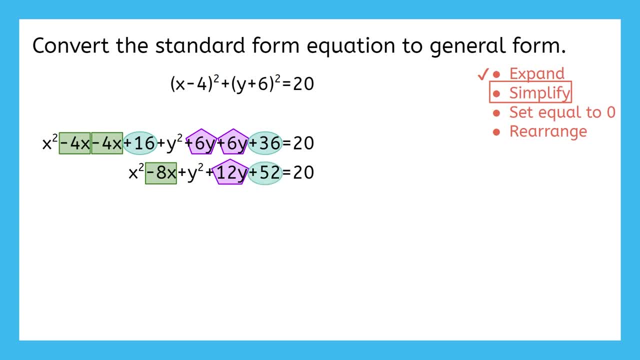 52.. Since there are no other x-squared or y-squared terms, those terms stay as they are, And we've now simplified as much as possible. Let's clear out some more space and move on to setting the equation equal to 0.. How can we get this equation to be equal to 0?? That's. 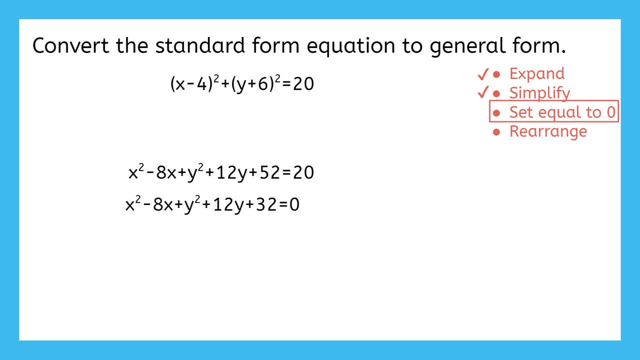 right. We can get rid of this 20 by subtracting it from both sides. We're almost done. Let's clear out some more space here. All that's left to do is rearrange our terms a bit so that they're in the right order. 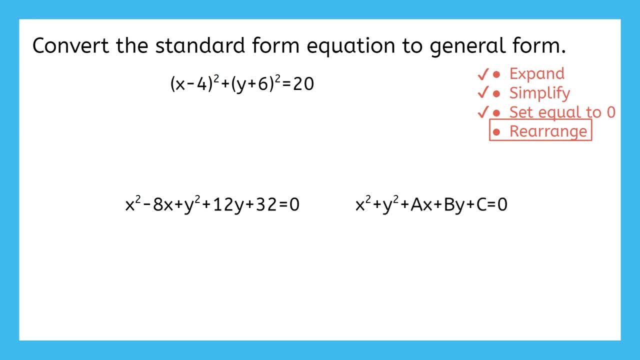 As a reminder, here is the general form circle equation. To be in general form, the x-squared term has to be equal to 0. In our equation, x-squared does come first, so so far we are on the right track. Next, 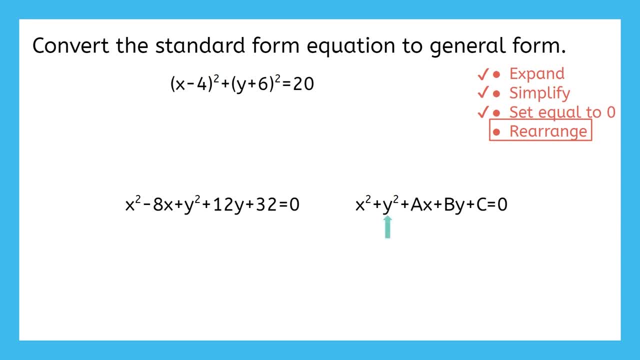 has to be the y-squared term. Ooh, our equation does not have the y-squared second. it has the x-term. That means we're gonna have to move the y-squared term over. Pause the video now and rewrite this equation with y-squared and minus 8x swapped. You should have written: 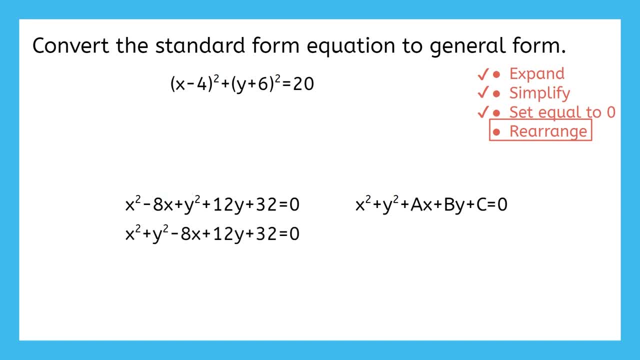 your equation like this: Now we have our y-squared term second, so let's keep going. We need to have the x-term third. Aha, Our little switch fixed this too. Perfect. Notice that it doesn't matter that this is. 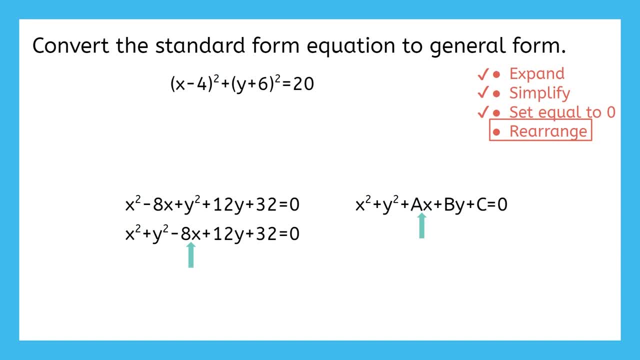 minus 8x instead of plus 8x. The operation does not have to be addition. Next, the y-term should come fourth. Yup, we have 12y here. And lastly, the constant term should be at the end of 4x. 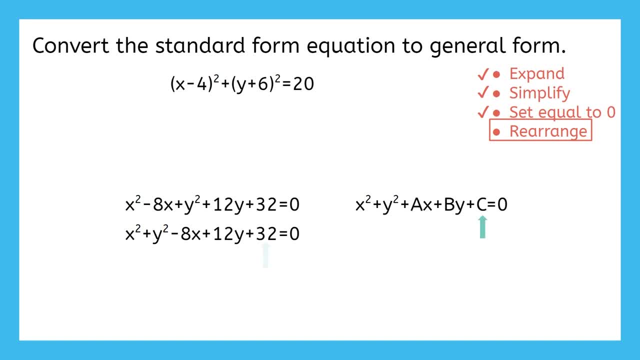 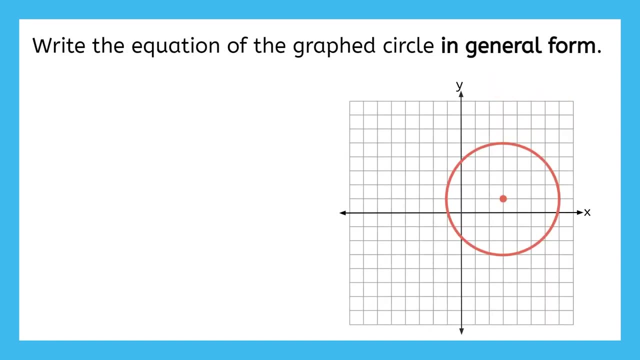 Bye of this part of the expression and, yes, we have 32 here. We have successfully rearranged our terms. so this is our final answer for the general form equation of this circle. This problem tells us to write the equation of the graphed circle in general form. 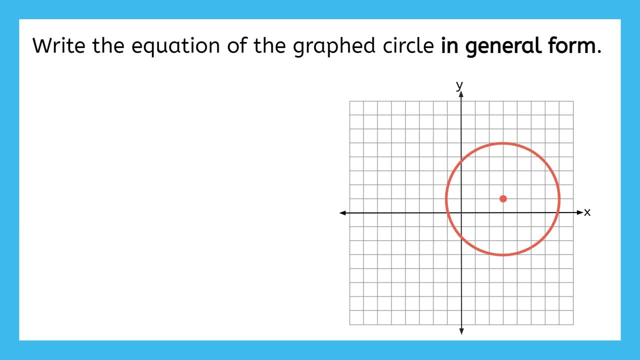 and we have a circle on a graph. Now we cannot just go straight from a graphed circle to writing its equation in general form. Instead, we're going to have to write the equation in standard form, using the center and radius first. Then we can go through all of the algebraic work. 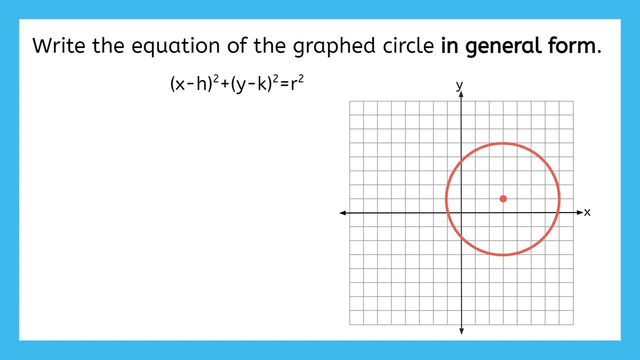 to convert it into general form. Pause the video here and write the equation of this circle in standard form. The center of this circle is at three comma one, so that means I can fill in h and k in my standard form equation. Luckily, if I move this circle, 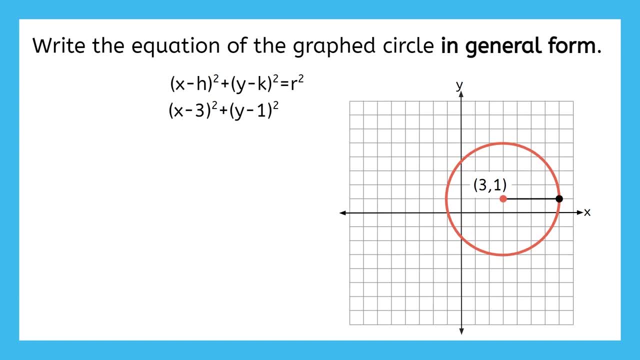 directly to the right of the center. the point on the circle falls on a whole number point, so I could just count and see that the radius is four units. You could also get the radius by moving up, left or down from the center instead of right. 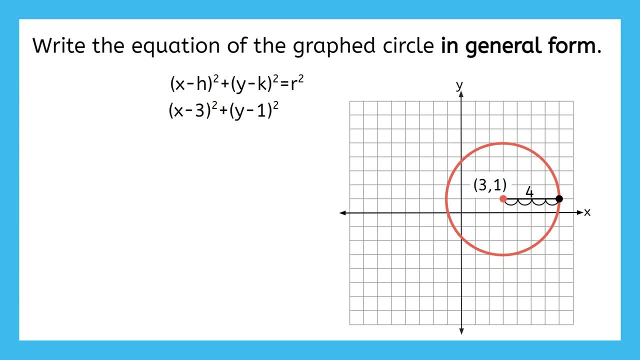 To put that radius into my equation: as r squared, that would be 16.. Now we have a standard form equation, so it's time to convert it into general form. I'll also get rid of this graph to give us some more room to work with. 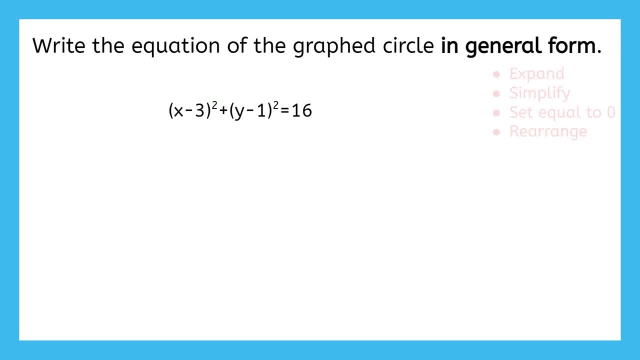 As a reminder to convert to general form, we're going to need to expand, simplify, set it equal to zero and then rearrange the terms. We'll start by expanding the equation. Pause the video here and expand this equation as much as possible. 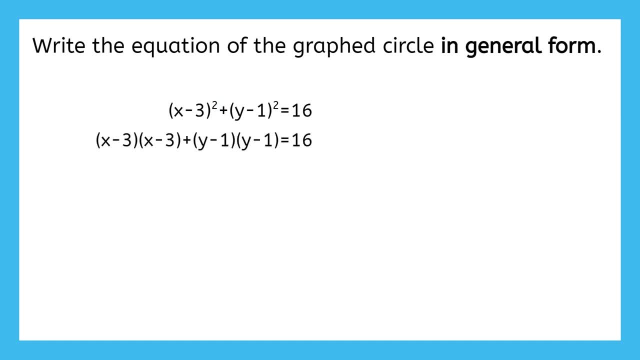 First I can write out the multiplication that my exponents are implying. Next, I can multiply both pairs of binomials: X minus three times x minus two times x minus three gives me this. And y minus one times y minus one gives me this: 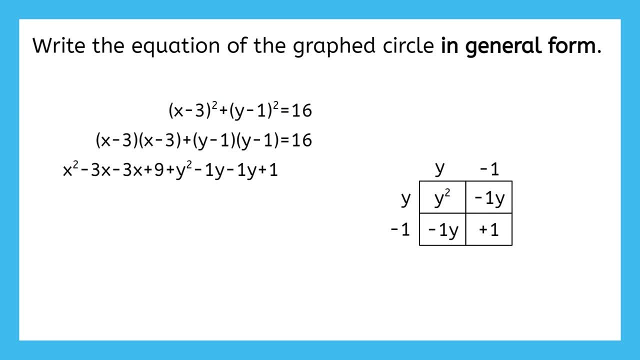 I've chosen to write these terms as minus one y, but if you left the one out and just wrote them as minus y, that is totally fine too. It's nothing to do with 16, so I just brought it down. After expanding, I need to start simplifying. 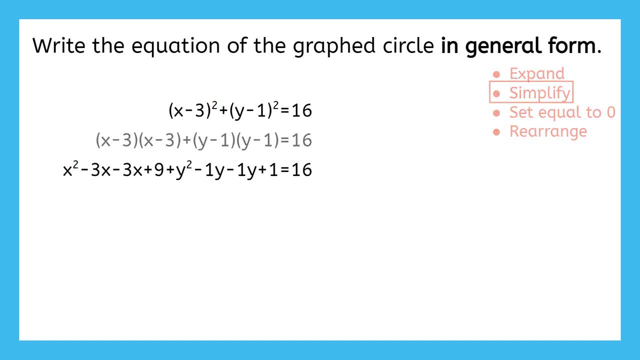 by bringing all of the like terms together. Let me clear up our workspace a bit. pause the video here and combine your like terms. I can combine my x terms to get minus 6x, my y terms to get minus 2x and my constants to get just plus 10.. So what should I do next? 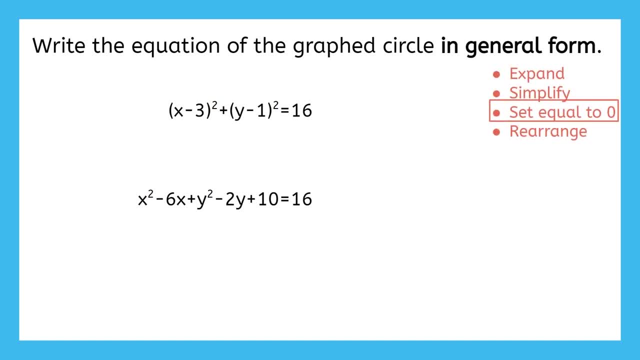 That's right. it's time to get this equation equal to zero. Pause the video and do that now. I can get this equation equal to zero by subtracting 16 from both sides. Is this a good final answer for the general form equation of a circle? 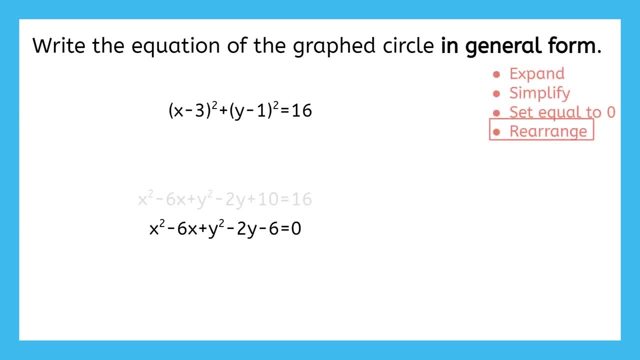 Nope, we're not quite there. We just need to rearrange our terms to make it match the general form equation. Pause the video now and rearrange your terms so that they're in the proper order. You should have swapped your y squared term and x term to get this. 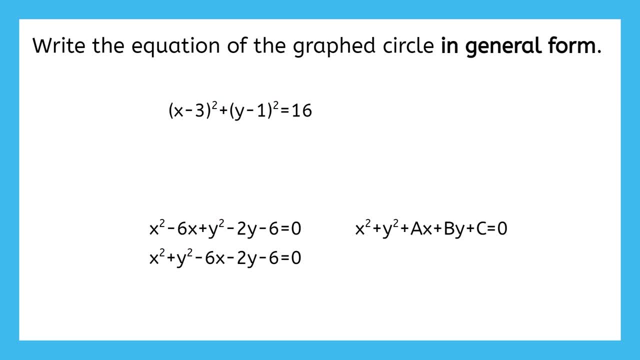 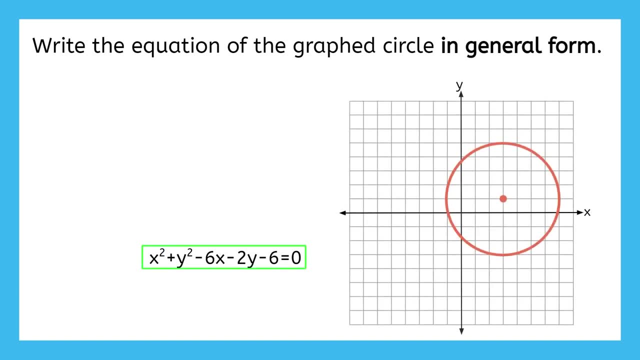 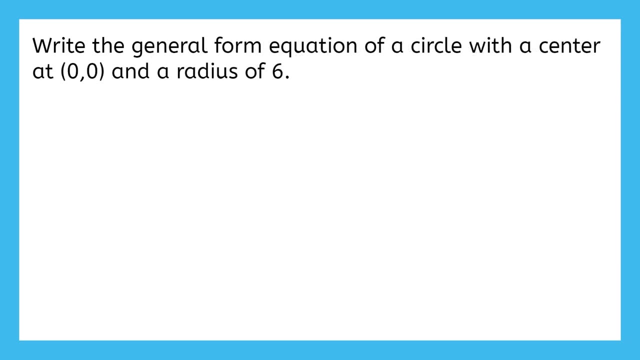 Again, I don't have to worry that I have a lot of subtraction in this equation instead of addition. The general form equation is all about the order of the terms, not their signs. All right, let's do one last example together. This problem says to write the general form equation of a circle with a center at: 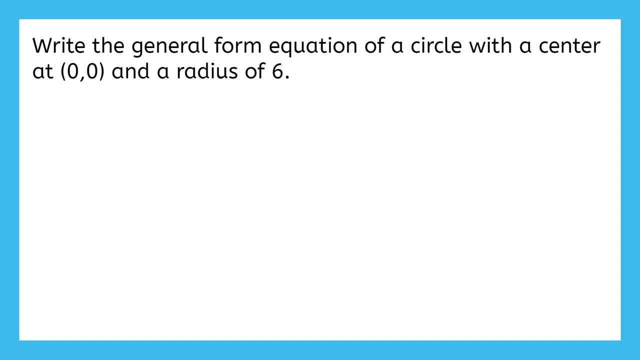 0, comma 0 and a radius of 6.. How should we start? You got it. First we need to write the standard form equation. So what does that look like? Since both h and k of the center are 0, that just looks like x squared plus y squared. 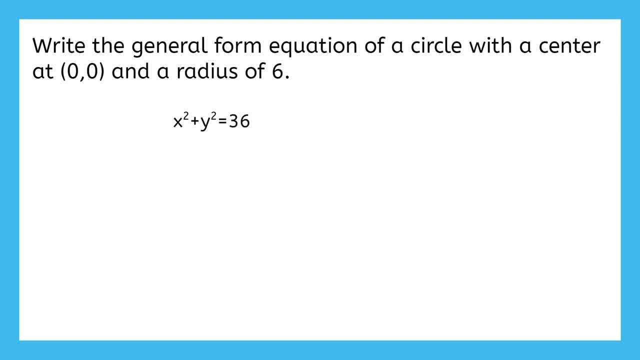 And since r is 6, r squared is 36.. Hmm, There's not actually anything here for me to expand or simplify. Can I set it equal to zero? Yes, I can do that by subtracting 36 from both sides.